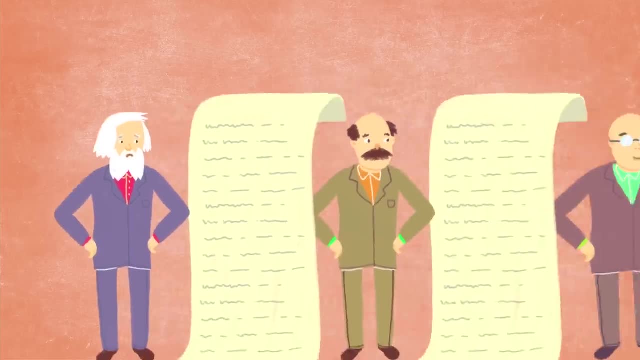 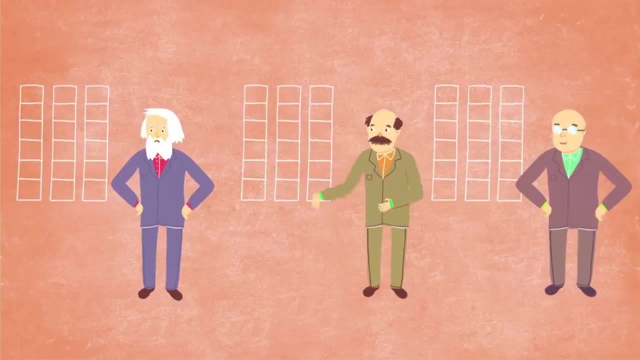 for making a list. Besides, Mendeleev was far from the first person to do that. Is it because Mendeleev arranged elements with similar properties together? Not really. That had already been done too. So what was Mendeleev's genius? Let's look at one of the first versions. 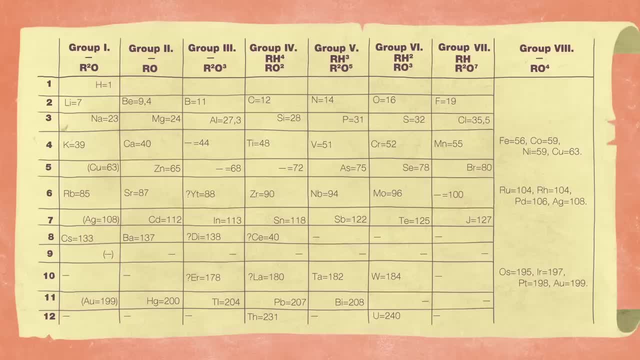 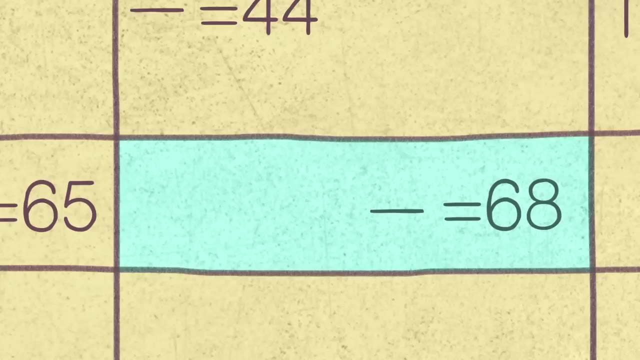 of the periodic table from around 1870.. Here we see elements designated by their two-letter symbols arranged in a table. Check out the entry at the third column, fifth row. There's a dash there. From that unassuming placeholder springs the raw brilliance of Mendeleev. That dash is science. 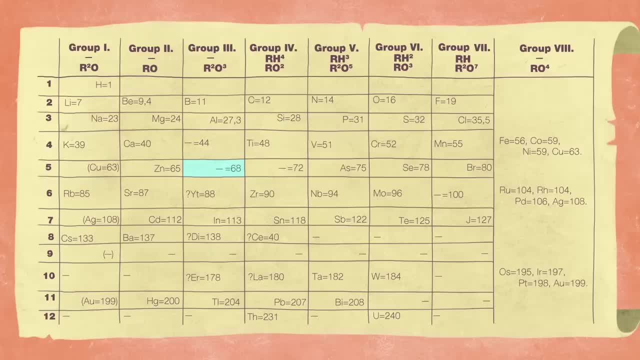 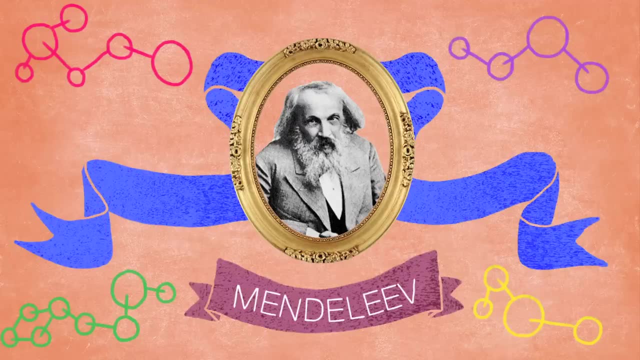 By putting that dash. there, Dmitry was making a bold statement. He said, and I'm paraphrasing here: y'all haven't discovered this element yet. In the meantime, I'm going to give it a name. It's one step away from aluminum, so we'll call it eca-aluminum, Eca being Sanskrit for one. 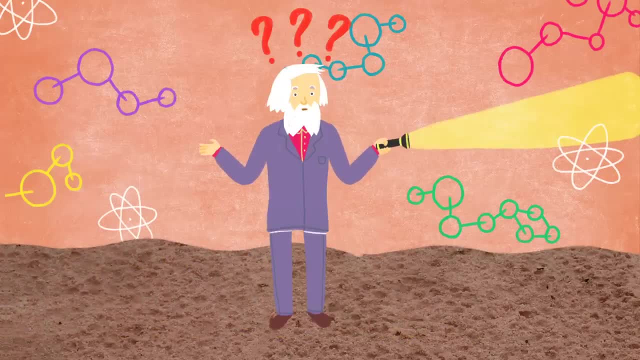 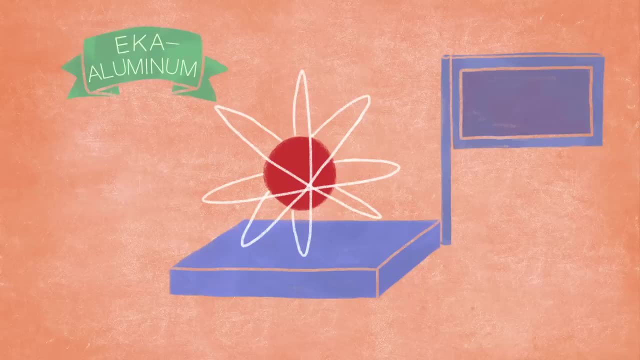 Nobody's found eca-aluminum yet, so we don't know anything about it, right Wrong, Based on where it's located. I can tell you all about it. First of all, an atom of eca-aluminum has an atomic 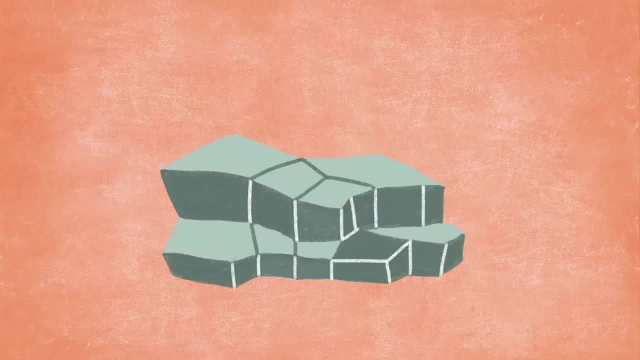 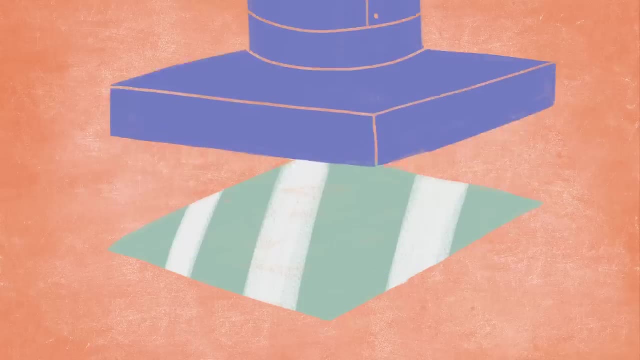 weight of 68, about 68 times heavier than a hydrogen atom. When eca-aluminum is isolated you'll see it's a solid metal. at room temperature It's shiny, it conducts heat really well. it can be flattened into a sheet, stretched into a wire, but its melting point is low. 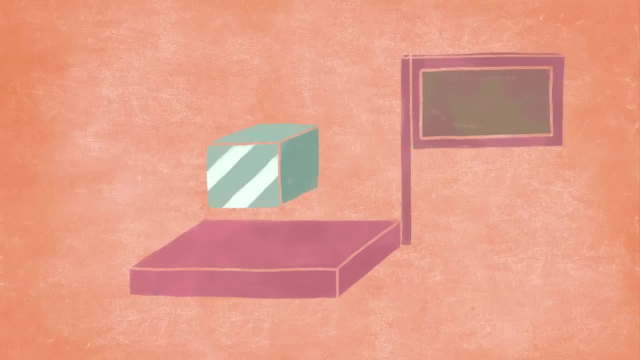 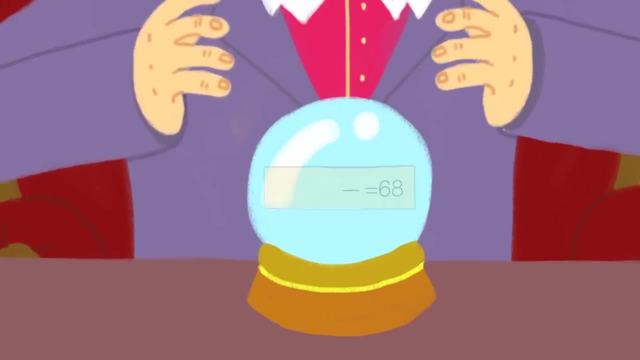 like freakishly low Oh, and a cubic centimeter of it will weigh six grams. Mendeleev could predict all of these things simply from where the blank spot was and his understanding of how the elements surrounding it behaved. A few years after this prediction, Mendeleev could predict the shape of 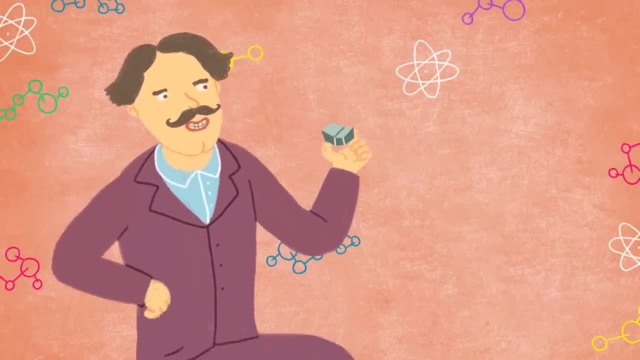 the atom and the shape of the atom itself. In the meantime, he could predict the shape of the gold and the shape of the aluminum. He could predict the shape of the silver atom and the shape of the aluminum. A French guy named Paul-Emile Lecoq de Bois-Baudrin discovered a new element in ore samples and 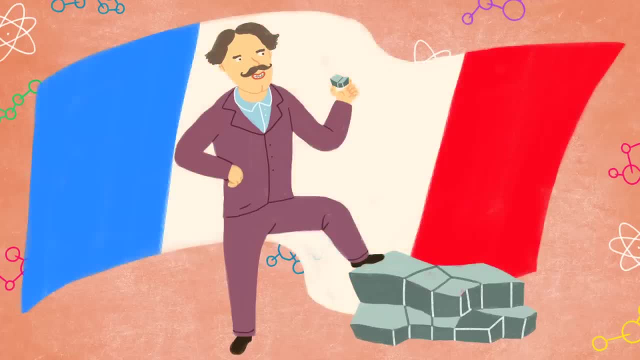 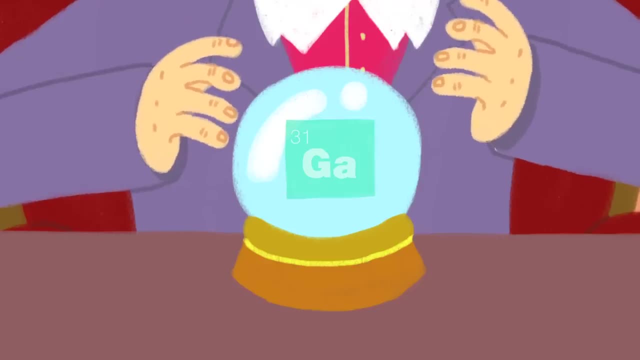 named it gallium after gall, the historical name for France. Gallium is one step away from aluminum. on the periodic table It's eca-aluminum. So were Mendeleev's predictions right. Gallium's atomic weight is 69.72..